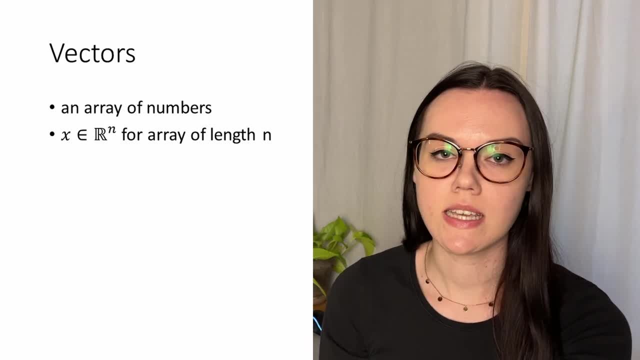 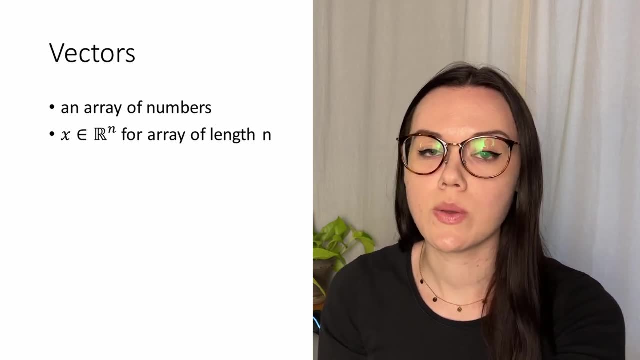 thing are vectors. A vector is basically just an array of numbers or a list of numbers, and you write it as x out of x, Of r to the power n, for example, if it's a vector of length n, And then if you want to show the 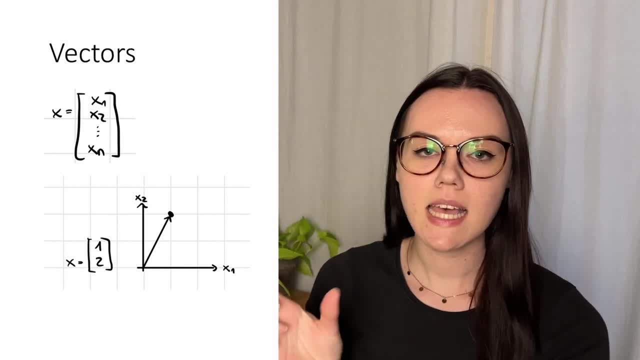 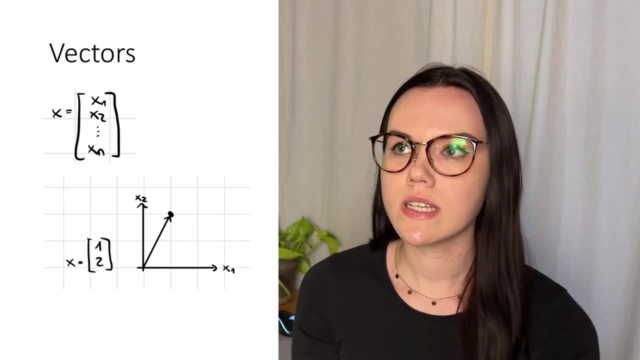 content of it. then oftentimes it's written as a column vector and then the elements inside of it are x1, x2, x3 and so on. An important difference to coding notation is that you don't use square brackets to access the different elements. Instead, you use a subscript, so you write a little one. 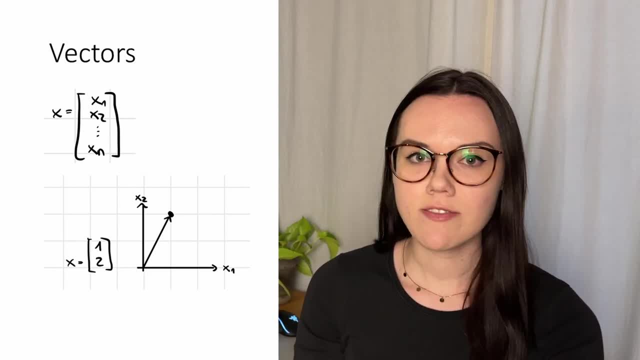 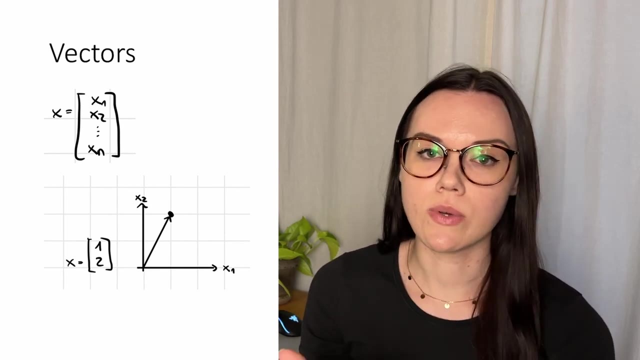 a little bit lower than the x. And importantly and kind of annoyingly to code math applications is that in math the first element is x1, whereas in programming the first element of an array usually is x and then square brackets zero, So you start counting at zero. 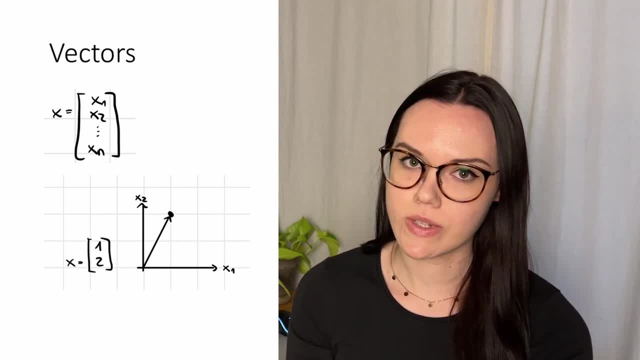 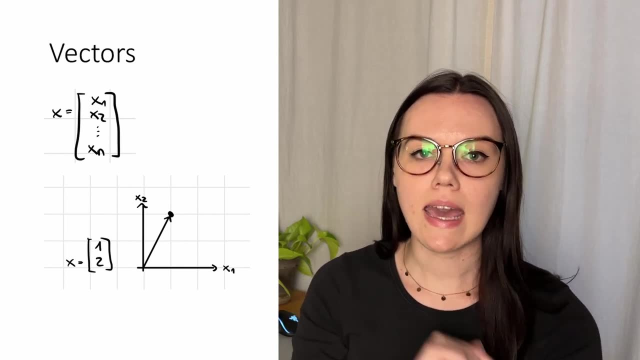 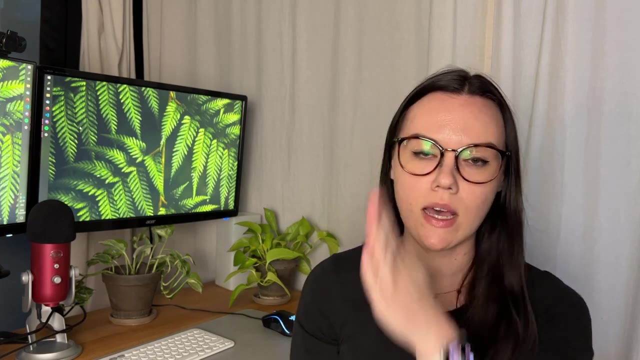 in coding and you start counting at one in math. usually, Depending on the context, you might imagine a vector as a point in space, or also an arrow to a point in space, like in this image here. Now, vectors were one-dimensional, so they only have one dimension of entries, but then the 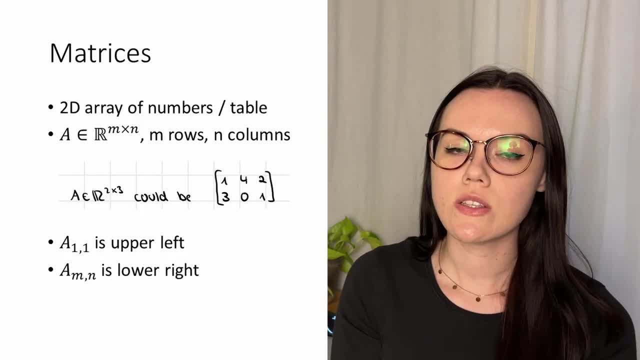 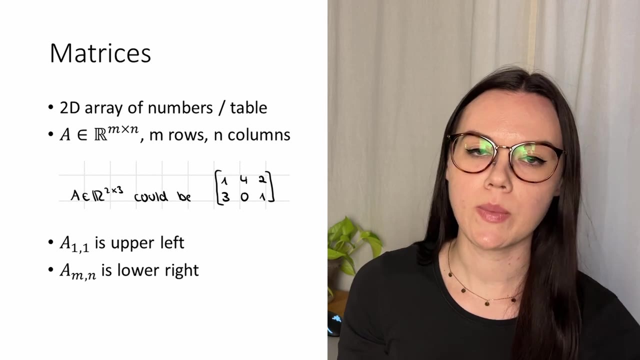 next step here are matrices. Matrices are two-dimensional arrays, or you could also look at them as a table of data. To write about a matrix in math notation you use uppercase letters like an- a, and you use r to the power of n times m for n rows and m columns. And here's an example. 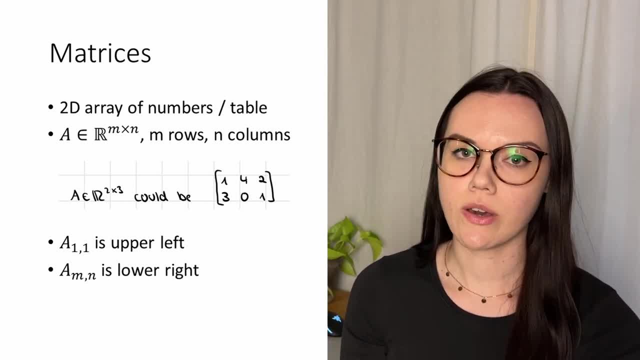 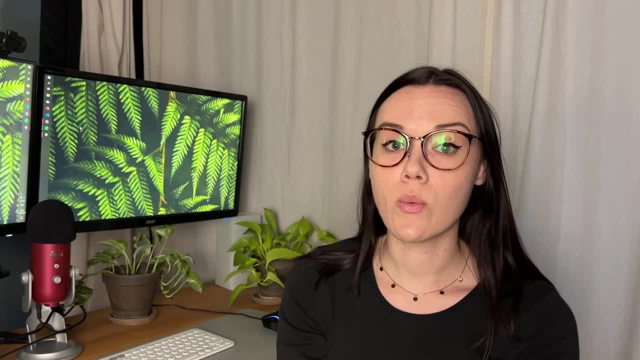 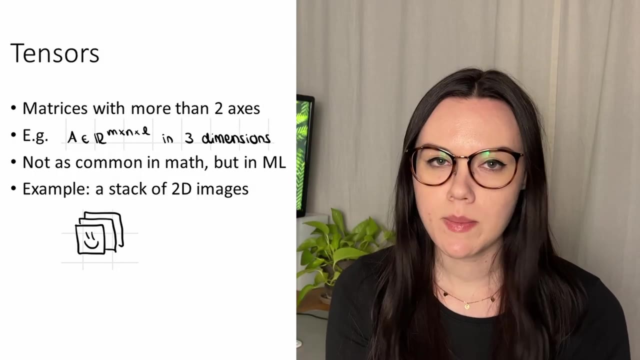 of a matrix with two rows and three columns. To index the elements, you again use subscript, but you index first the rows and then the columns. But what if you have more than two dimensions? Well, that's where tensors come in. So tensors are basically just the same thing as a matrix, but 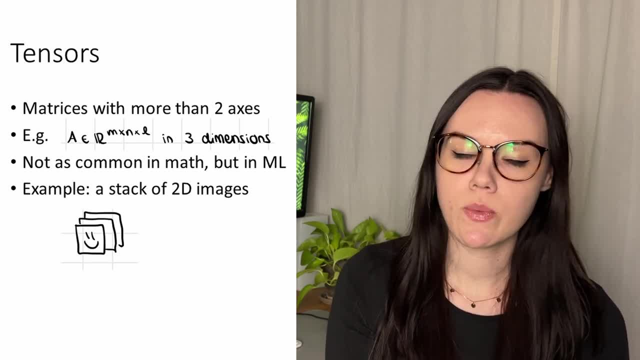 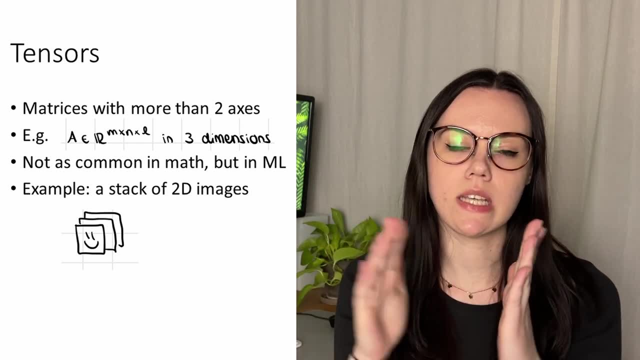 with three or more dimensions. You use the same notation with an uppercase letter and then in the exponent you say the different dimensions and like how large each dimension is, So n rows, m columns and then l stacks or however else you want to imagine the third dimension. 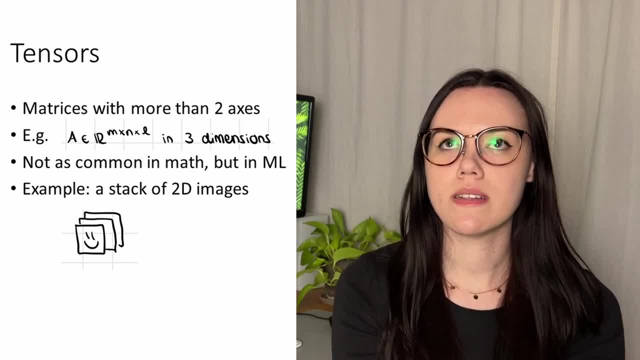 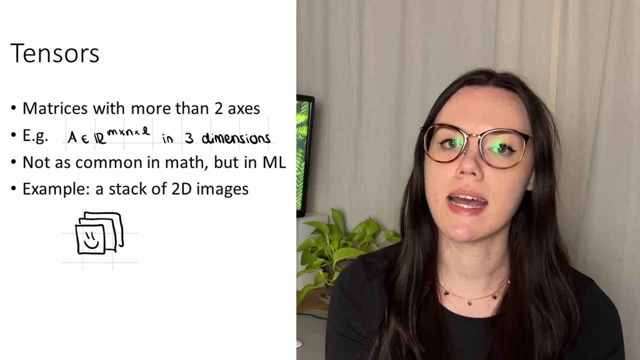 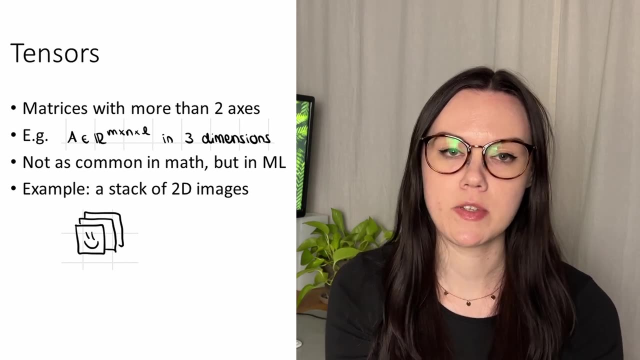 Tensors are not really a math thing, but they are very common in machine learning, especially deep learning. In deep learning libraries like pytorch or tensorflow, as the name already implies, most of the data that you save will be in the form of a tensor object, And a very great example. 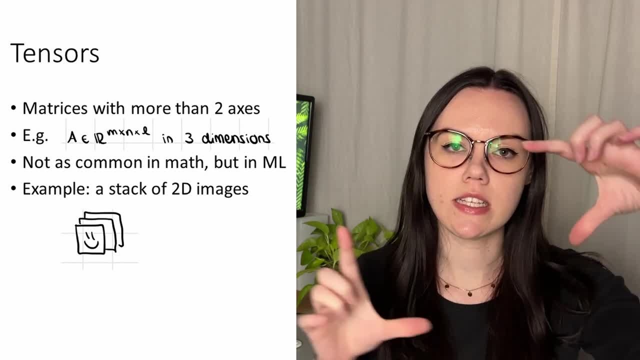 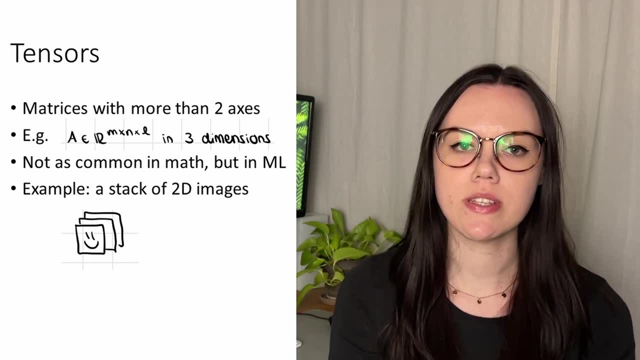 is a stack of images. So in a stack of images you have a stack of images. So in a stack of images you have an image that is two, two-dimensional in nature, So you have like a height and a width, and then there are pixels inside of it. so that's two dimensions. And then the third dimension of 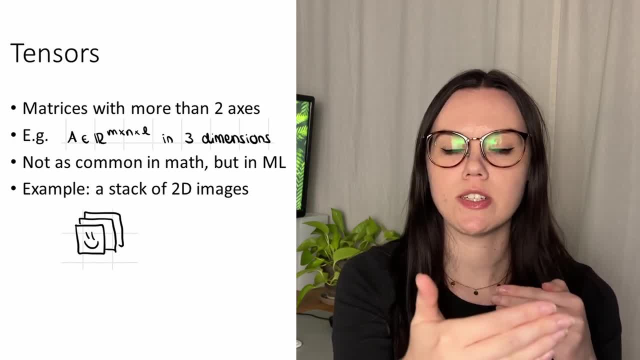 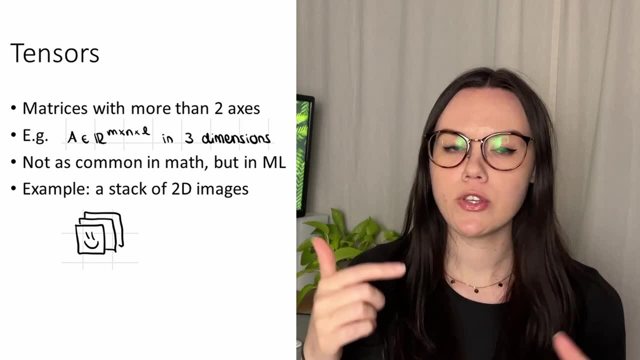 a tensor of data would be that it's multiple images at the same time, So you can imagine it as a stack of papers. If you would print them out and stack them on top of each other, they would form a cube right, So like it's a two-dimensional image and then you have multiple. 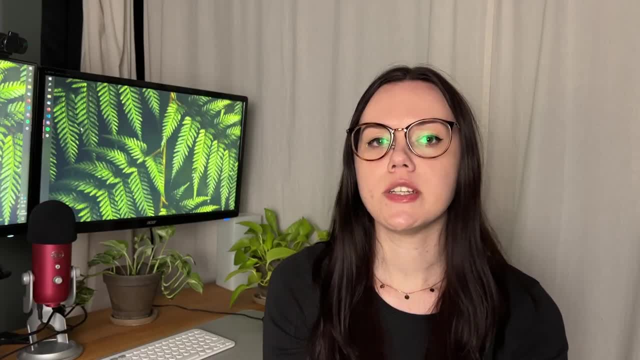 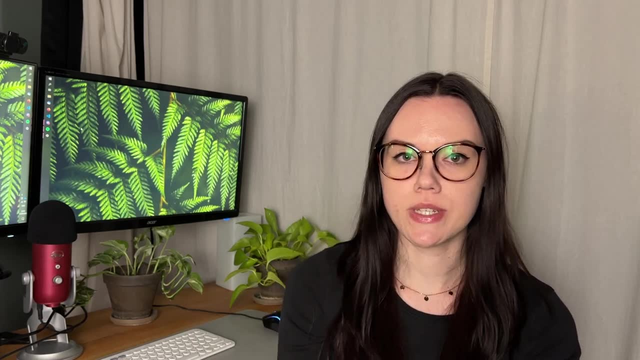 of them. so that's the third dimension And you use stacks of images or like groups of data in general To pass them through a neural network at once, to use parallel computing. But really the key takeaway here for linear algebra are matrices, because basically tensors- 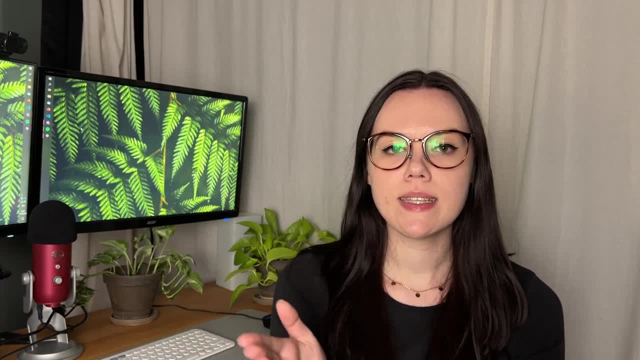 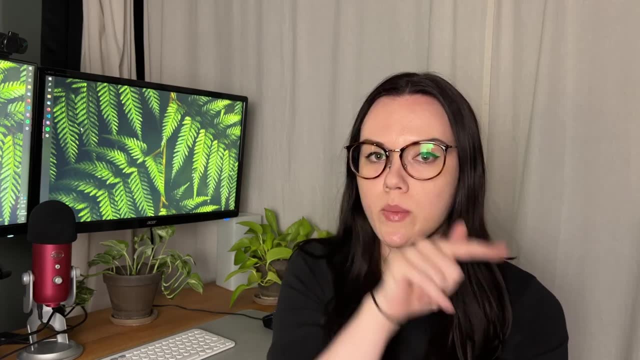 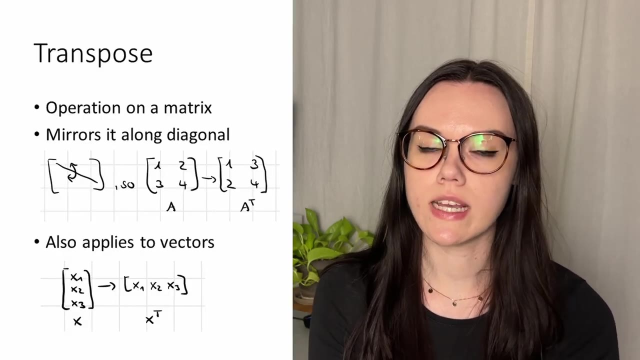 are just matrices with an extra dimension. Vectors are just one-dimensional matrices and even scalars, the single number- you can think about them as a one by one matrix. So let's look at some important operations on matrices. One of those key operations is: 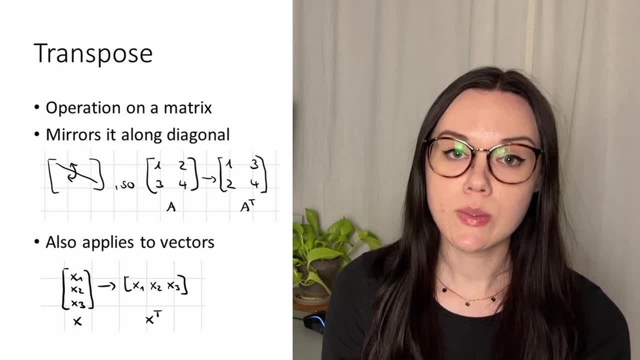 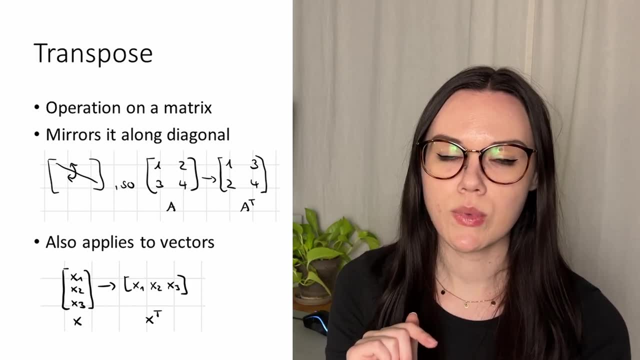 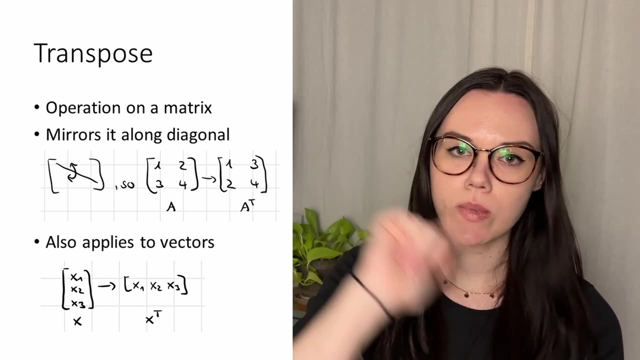 the transpose or transposing a matrix. Transposing a matrix means mirroring it along its main diagonal. Here on the side is an example where you can see that the main diagonal stays the same. the one and the four and then the two and three chains change their spots because you fix the diagonal. 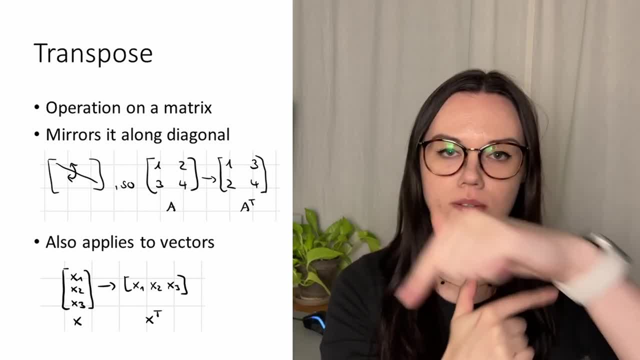 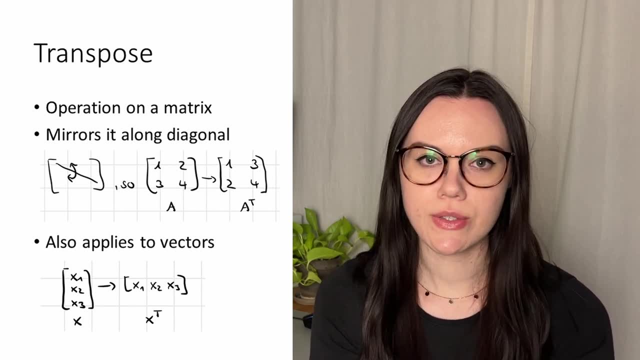 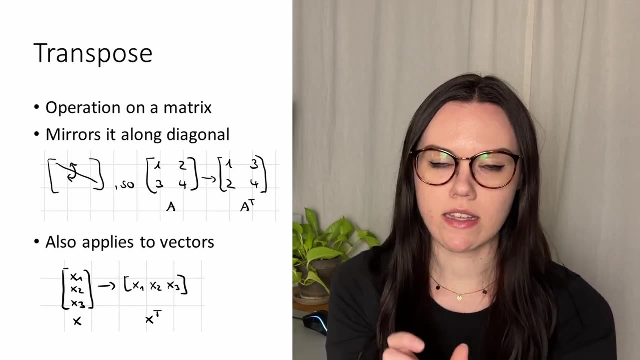 and then everything on the sides gets flipped around. You can also apply this operation to a vector. So if you have a column vector and you can also apply the transpose to a vector, If you start out with a column vector and you then flip it along the diagonal, it doesn't really have a diagonal, so you only 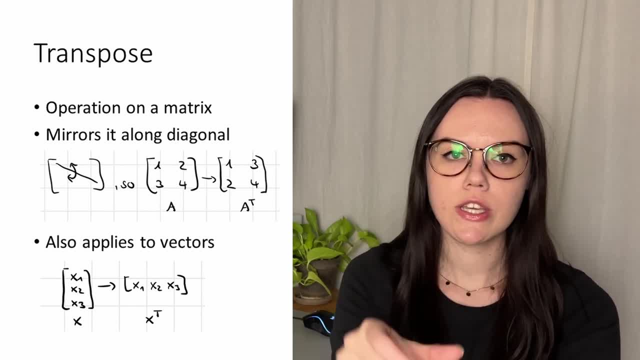 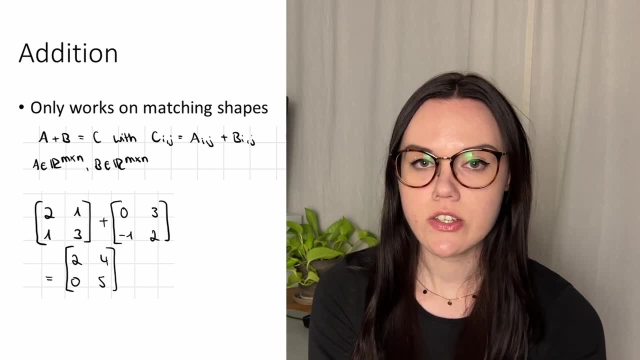 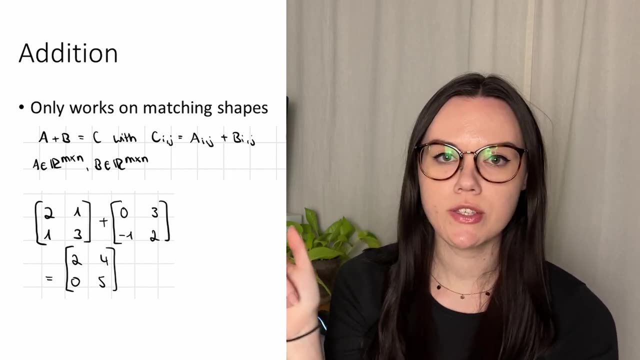 fix the top entry and then you flip it from downwards to the side and then you have a row vector. The next key operation is addition, and addition of matrices only works in theory if they have the same shape. So if it's a two by two and a two by two, you can add them up. 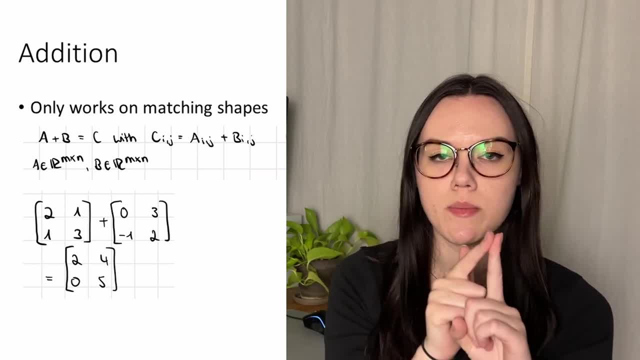 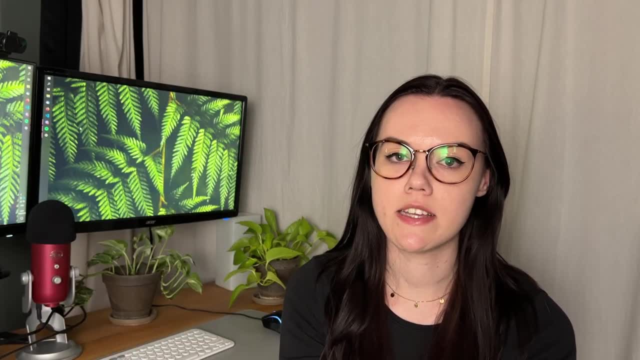 entry wise, So if you take the top left of each and add those numbers together, and then you take the lower left and add those two together, and so on. Of course there's also matrix multiplication, but the process of that is a bit more difficult, so I'll save that for another video. 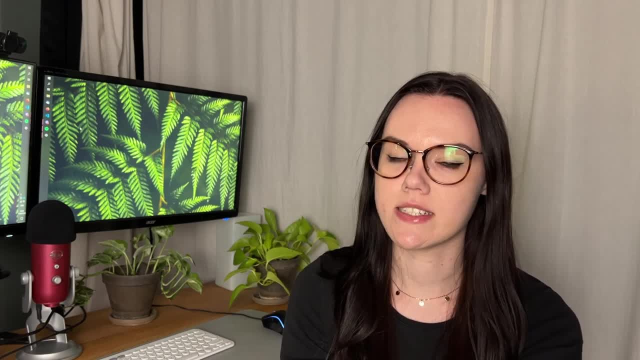 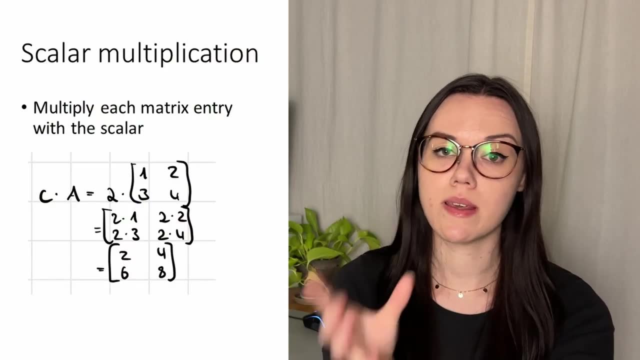 But what we can talk about is scalar multiplication, and that's where the scalar from the start of this video comes in. Scalar multiplication means you take a number and multiply it with a matrix, and in that case you multiply the scalar with the though division. No, I'm sorry, this is the wrong way to say this. If you take a second matrix, you get a second. matrix, so hide the first step so you save that for another video. Here we have an example of simplification: The wholeấu Reduce to two by two and then multiply them by a matrix and end up with a second matrix in order to find the various законs. cannot be. 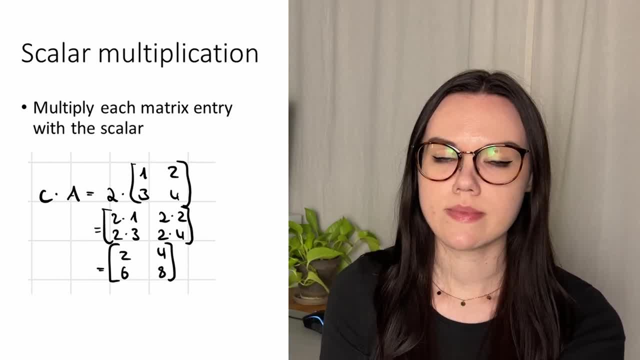 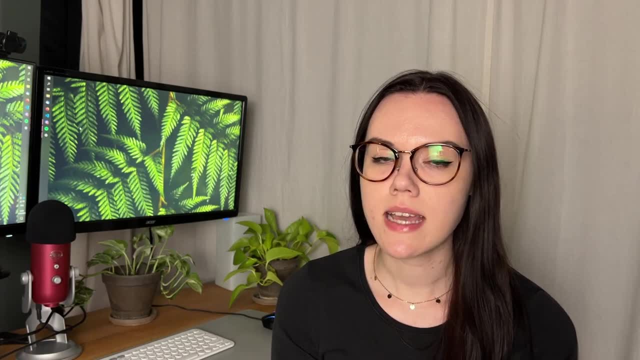 scalar with each of the entries in the matrix separately, And then the end result will be another matrix of the same shape as the original matrix. Now, when talking about addition, I just mentioned that the two matrices have to have the same shape or the same dimensions. But in many 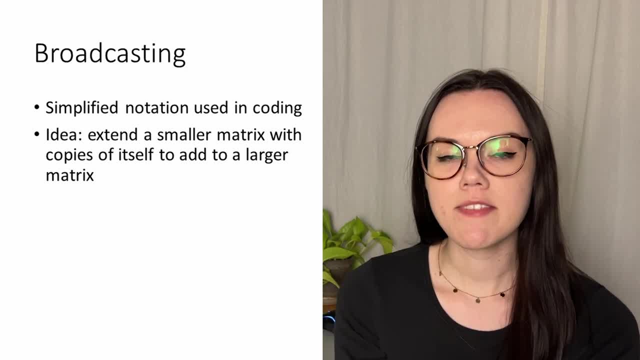 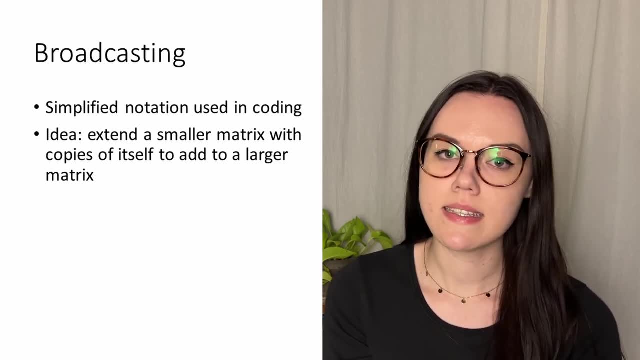 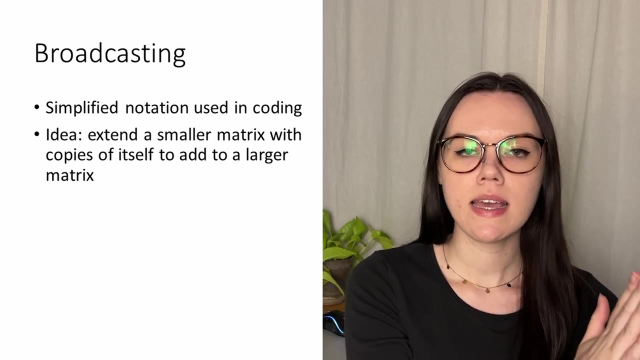 programming languages like Python. there is some simplified notation that they implemented, so you can add matrices together, even if they have different shapes. The idea here is to add a smaller matrix, or even a vector, to a larger one by taking the smaller one and duplicating it next. 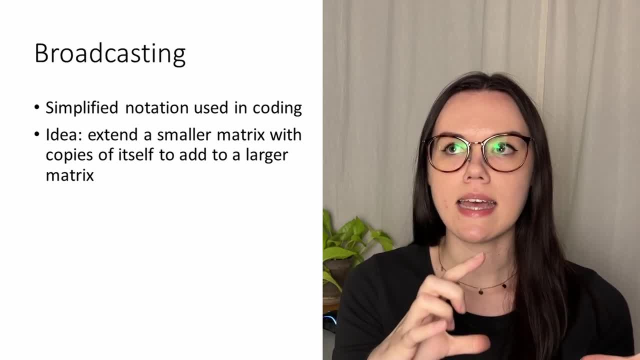 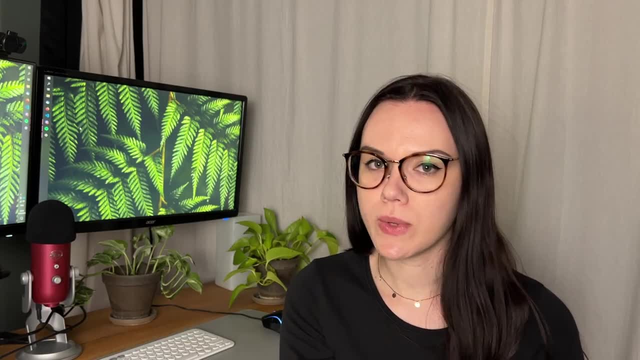 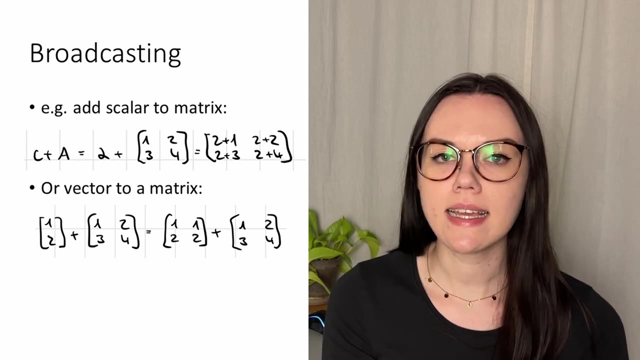 to each other, and then creating a matrix that has the same component over and over again until it matches the bigger one. Now, that might sound a little weird at first, so let's look at an example. One way to do this is you could add a scalar to a matrix and in that case, the scalar the one. 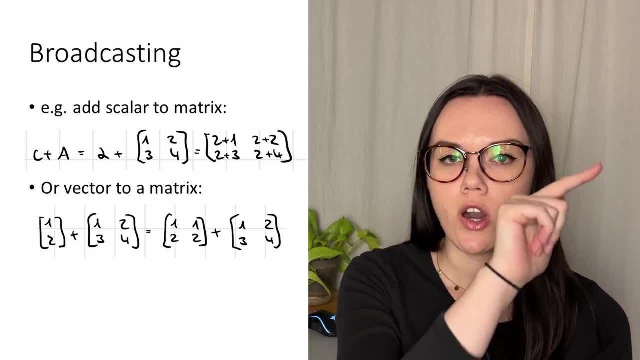 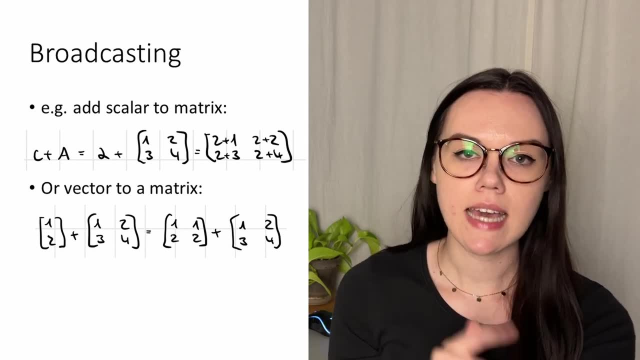 number. if you add it to a two by two matrix, it will be copied until it will be added to each entry of the matrix separately. Now I've written the end result here, but you can imagine that in a step in between the two will be extended to a two by two. 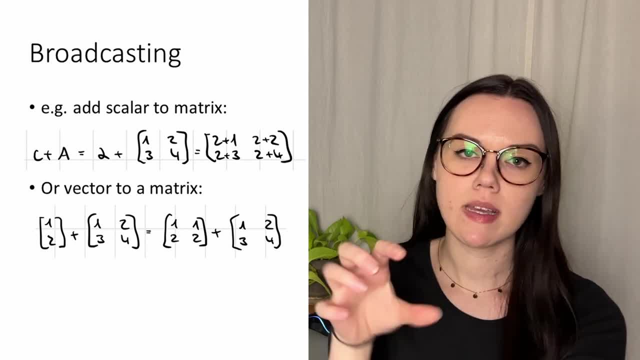 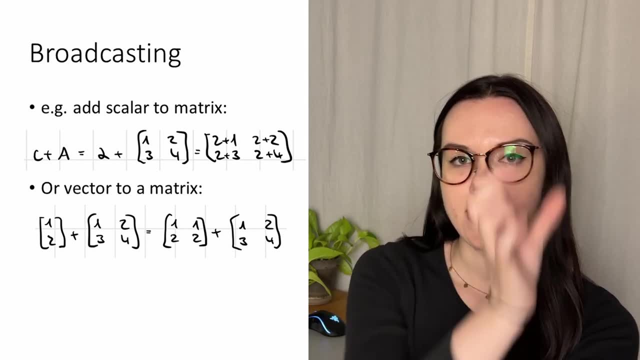 matrix that is just full of twos, and then the two matrices can be added. normally, A very common application of this in programming is if you add a vector to a matrix and both of these have the same number of rows, but of course the vector only has one number. So if you add a vector to a matrix,